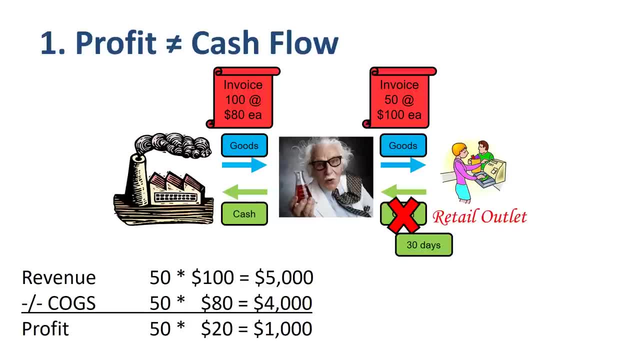 How much cash flow do you generate? Well, you don't get paid by the retailer until one month from now, so cash in is zero. You paid your supplier on delivery, so cash out is $8,000.. Total cash flow is negative $8,000. 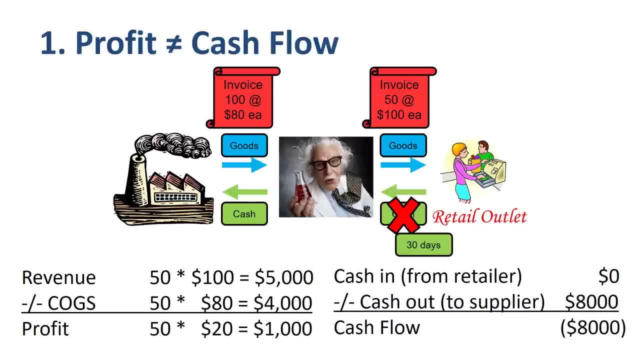 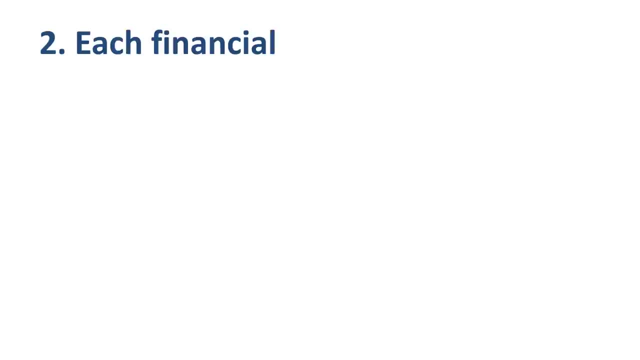 Profit on your shipment is recognized when you deliver the goods to your customer, the retailer. Cash flow is recognized when cash comes in or cash flows out. You could be profitable yet go bankrupt. Finance idea number 2.. Each financial statement tells a story. 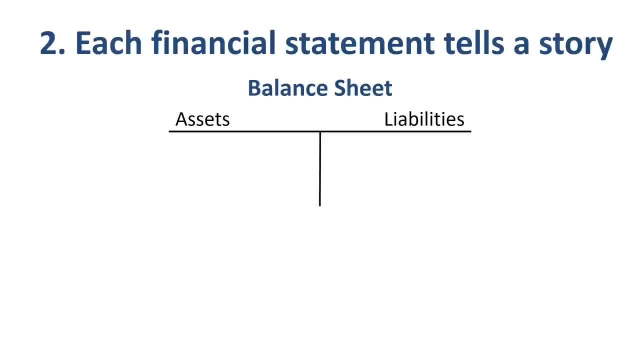 The balance sheet gives you an overview of assets, liabilities and equity. It shows what we own on the left and what we owe on the right. The income statement tells you what you owe. The income statement shows you how revenue minus expenses equals profit or loss. 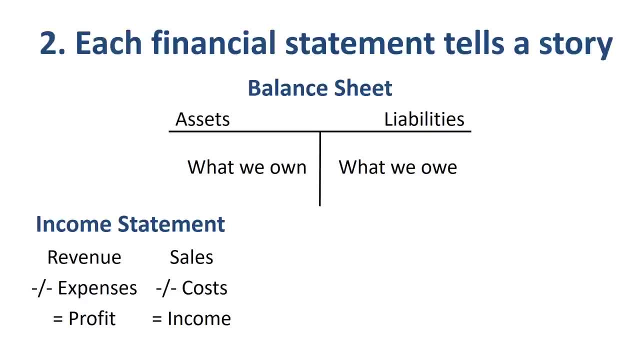 Or in other words, how sales minus costs equals income or loss. The cash flow statement shows you how you got from the cash balance at the start of the year, through cash inflows and cash outflows during the year, to the cash balance at the. 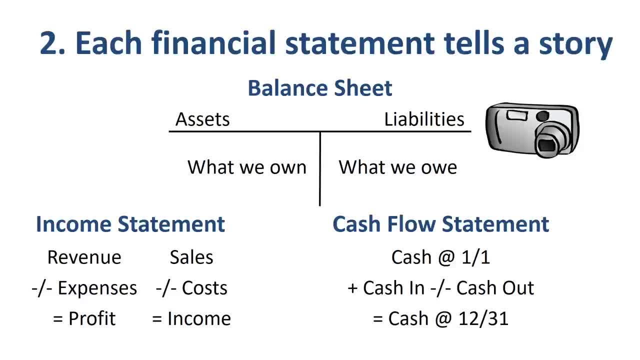 end of the year. A balance sheet is a picture at a point in time, usually the end of the month, end of the quarter or end of the year. An income statement is a picture of the balance sheet. A balance sheet is a picture of the balance sheet. 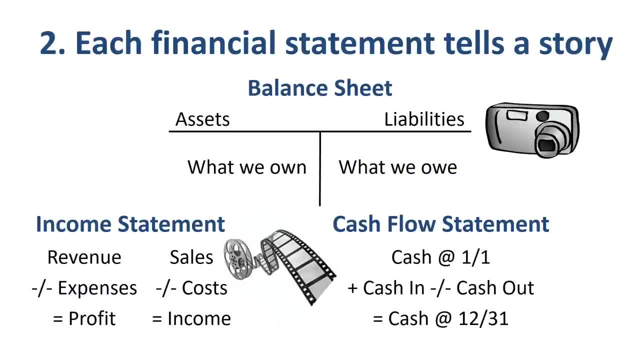 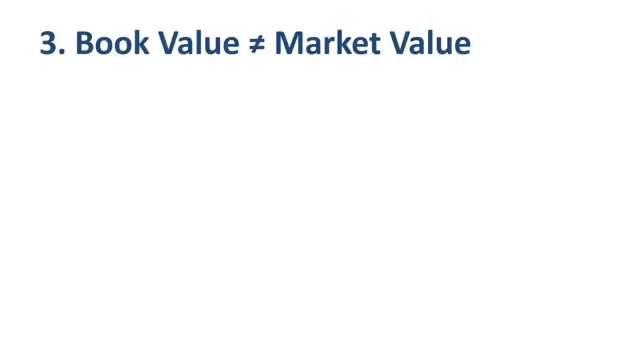 A cash flow statement is a movie of profitability during a month, quarter or a year. A cash flow statement is a documentary movie about movements in the most fascinating account on the balance sheet. cash Finance idea number 3. Book value- what a company is worth on paper, based on the balance sheet, is not necessarily. 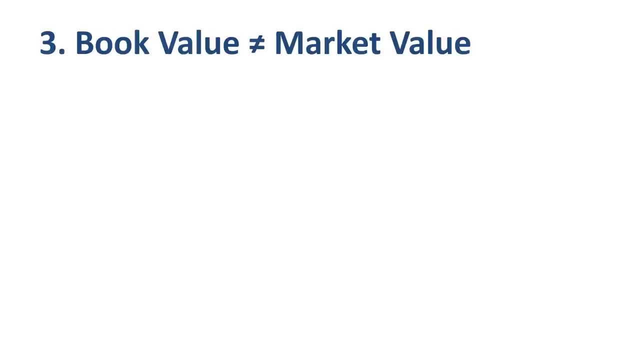 the same as market value what someone is willing to pay for it. Let's look at Apple Inc. The book value of its equity on the balance sheet of market value is not necessarily the same as the share price. The share price of March 30, 2019 is around $106 billion. 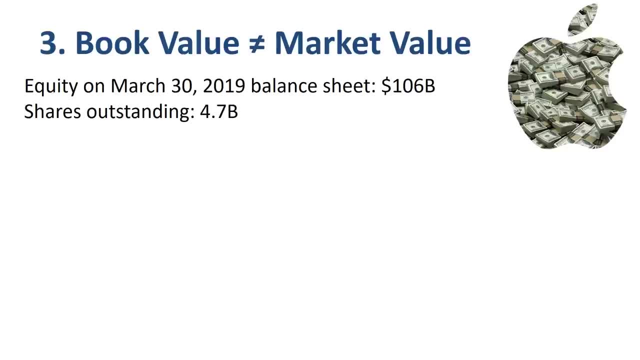 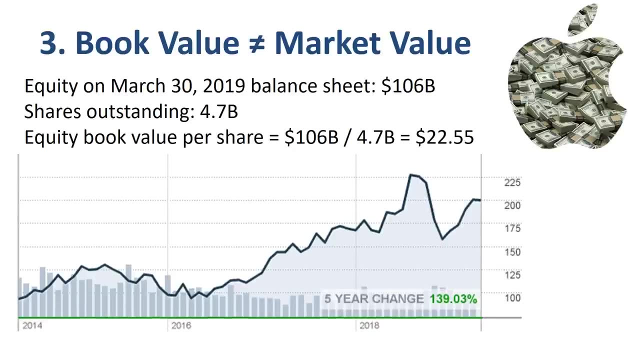 The number of outstanding shares 4.7 billion units, so the book value per share is around $22.55.. If you look at the market value of the share price in early May 2019, you see the share price around $200. 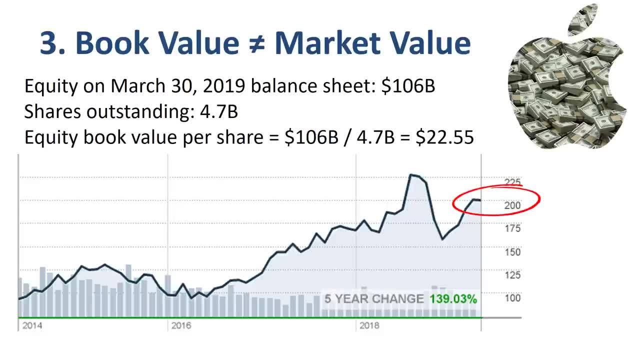 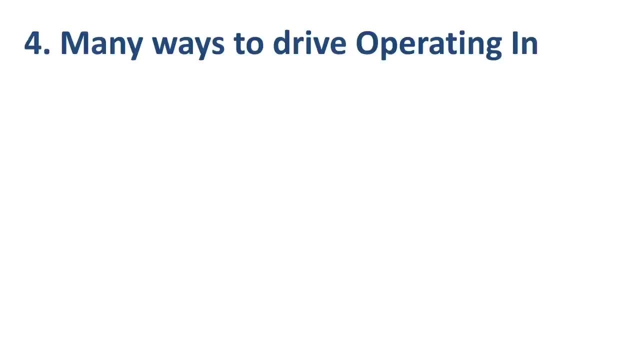 Book value or accounting value is based on the company's historical financial results. looking back, Market value or economic value depends on the expectations of investors for the future of the company. looking forward: Finance idea number 4.. There are many ways to drive operating income. 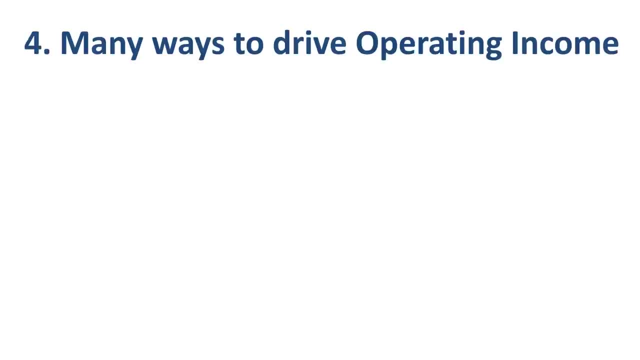 If you listen to CEOs and CFOs, it sometimes seems that the only thing they can think of is cost cutting, cost cutting and more cost cutting. While that could certainly be an appropriate way forward, there are more options to choose from. Price: 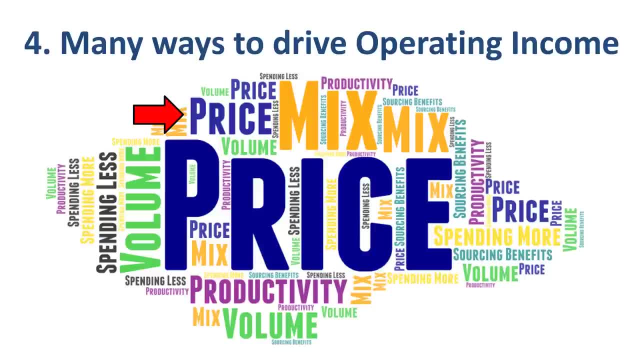 Are you charging a price to your customers for your goods and services that accurately reflects the value you are creating for them? Volume: What opportunities do you have to sell more units? Mix: Can you focus more resources on selling the higher margin products and services in your 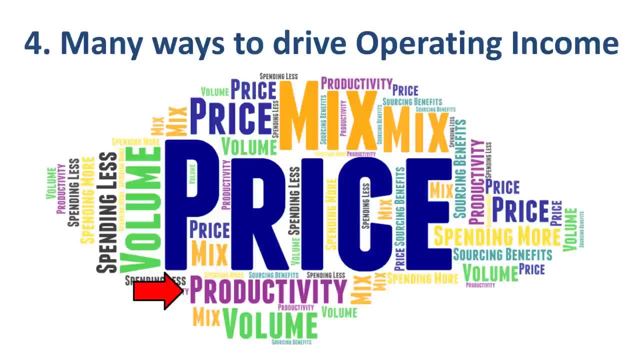 portfolio versus the lower margin ones? Productivity: Can you generate the same amount of output with fewer resources or more output with the same amount of resources? Sourcing benefits: Can you renegotiate your contract with your existing suppliers to get lower price or more? 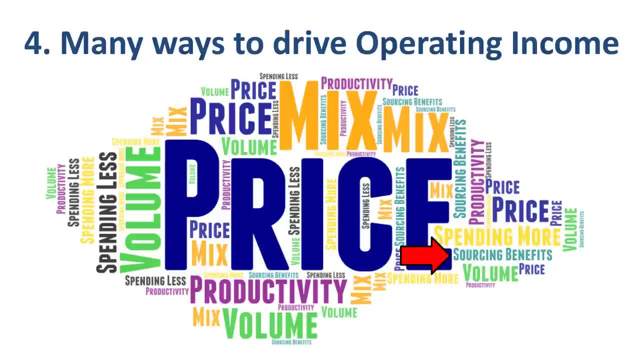 value, or can you find alternative suppliers that give you a better deal Spending more? Can you spend more on research and development to develop your product or service faster and better and generate more revenue and margin? Can you spend more on marketing to establish your brand? can you spend more on learning? 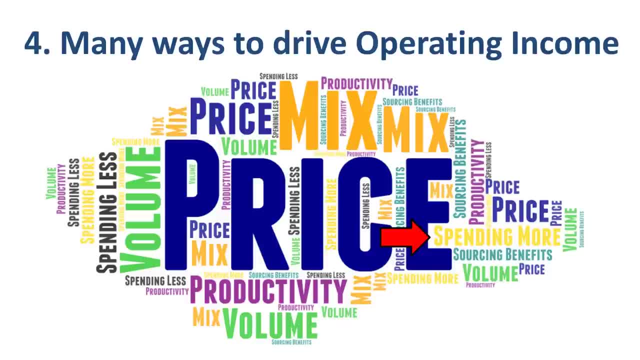 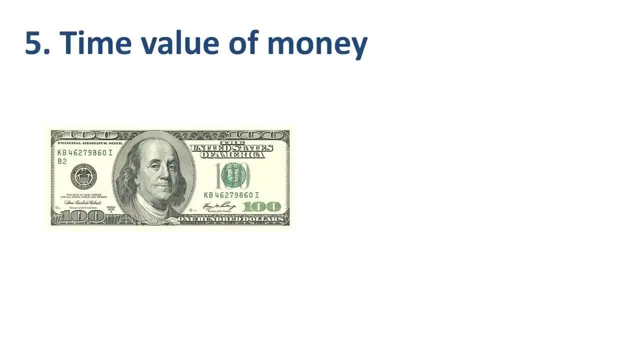 and development to improve the skills of your customers. Sourcing benefits. Can you keep up with your employees? Finance idea number 5.. It's your lucky day. Somebody wants to give you $100.. Would you like to receive that $100 right now, today? 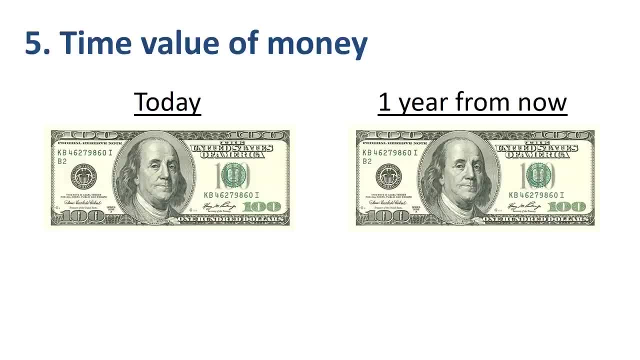 Or would you like it one year from now? I'm pretty certain you would say $100 today. All sorts of things could happen during a year, right, Mr? Somebody might change his mind about giving you the money. Mr. Somebody could go bankrupt and be unable to give you the money. 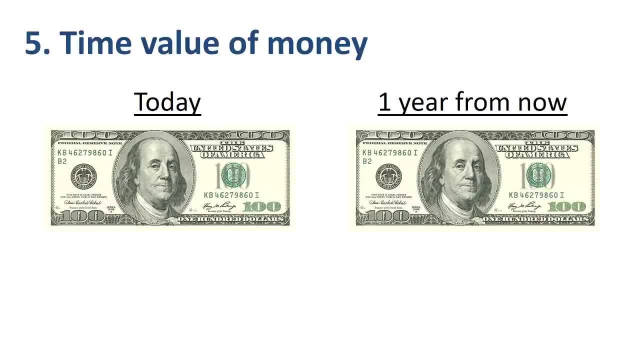 Mr, Somebody could go bankrupt and be unable to give you the money, could be inflation that decreases the purchasing power of the $100 you receive. That's the idea of time value of money. $100 today is not the same as $100 one year from now.